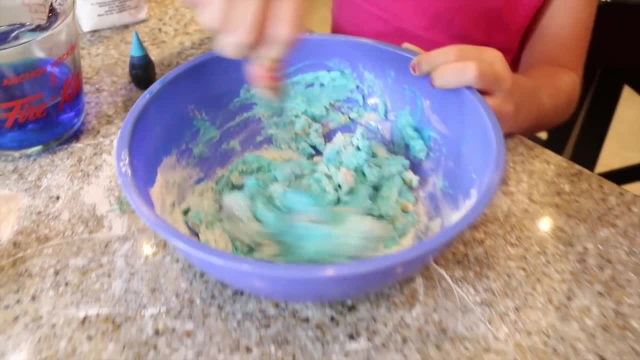 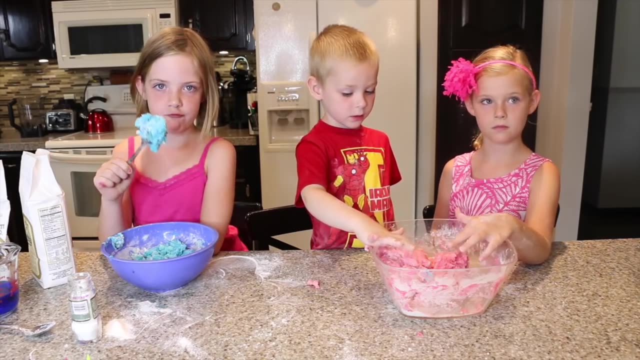 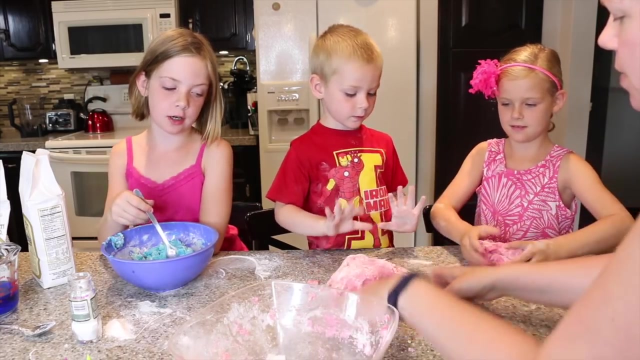 So we've added the water until we get a nice sticky paste. Now the most important part is kneading it. So you dump it out of your bowl. We're going to break it into two, One for each of them, And Brad's going to like that And we're going to. we're going to knead. 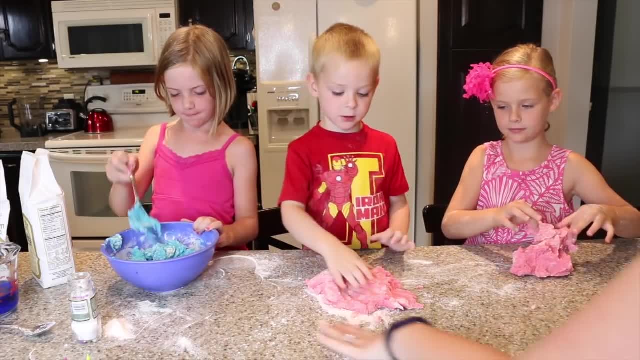 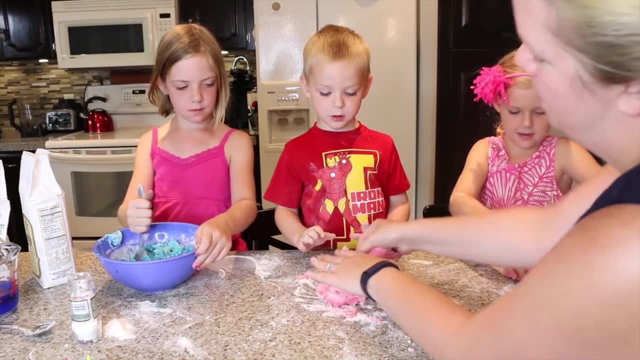 it. So kneading it means you're just, it's warm. You want to let it cool. We let ours cool a little bit, but it's still warm. You want to knead it just by turning it over and and pressing it And playing with it, And playing with it, Exactly So dump yours out. 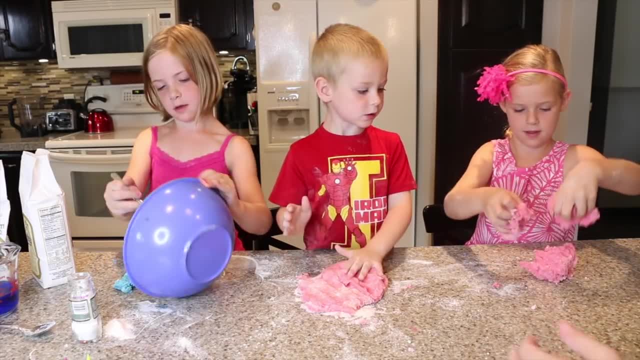 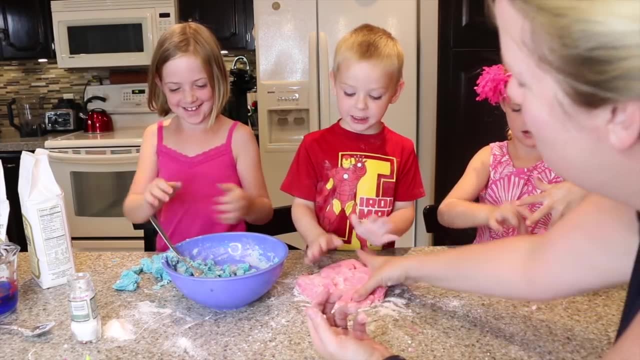 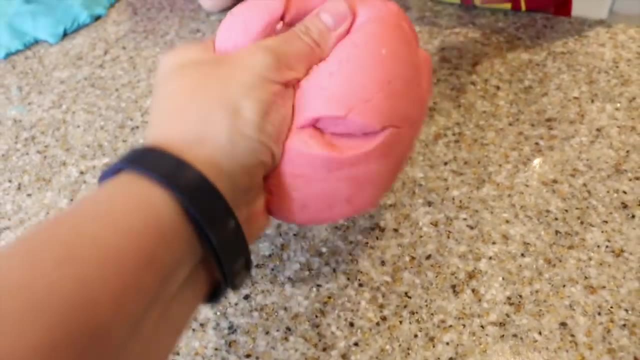 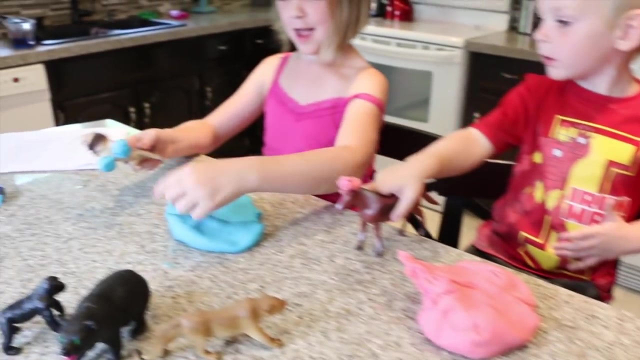 Izzy and play with it until it's the perfect consistency. If it's still feeling a little bit sticky, you're going to want to add some more flour. Yes, Now he's really good at it. He's really the king of the jungle. That's nice. What is that? His shoes. 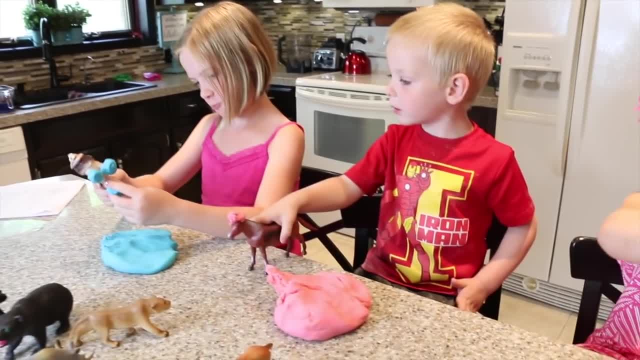 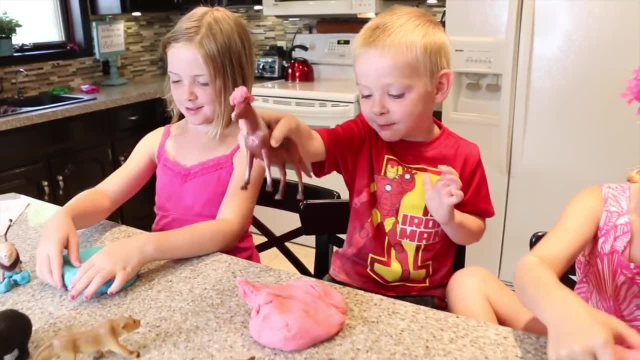 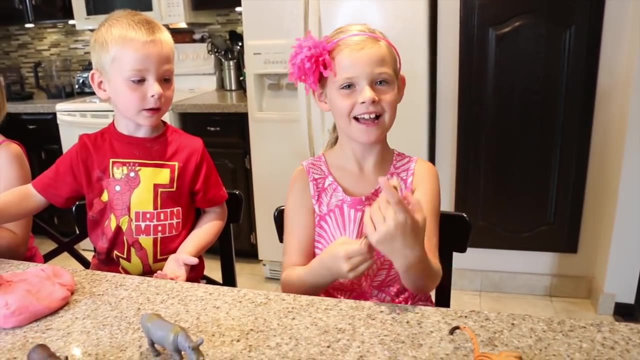 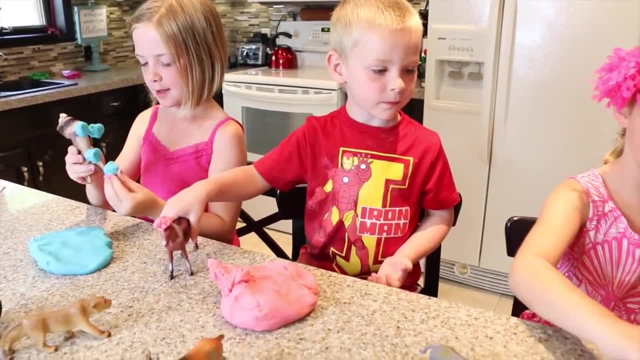 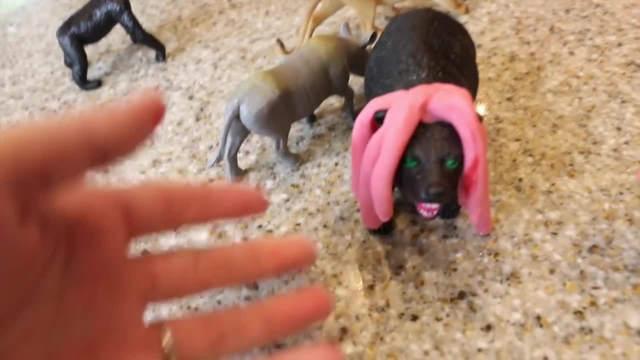 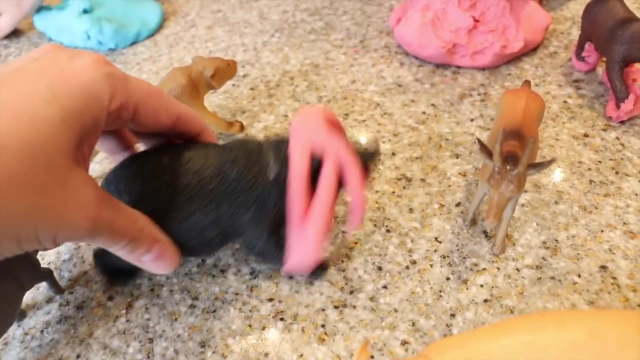 Her clothes? She can't be, she can't be naked. Who's this Making her shoes? I made my bear a nice hairdo. What do you think? Yeah, great, Can I see This lion takes so much precaution. 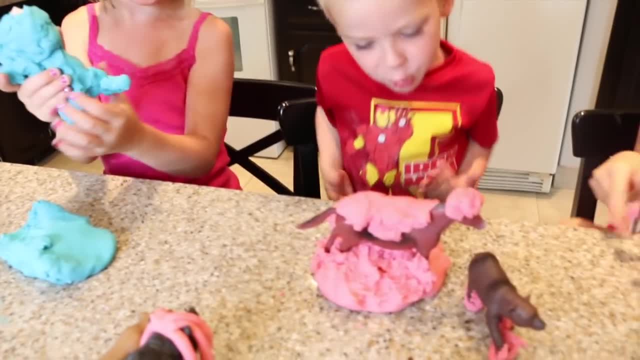 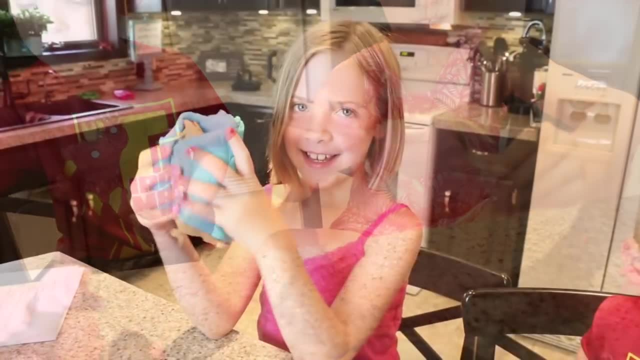 I am a cool dog, dude. Look at my beautiful deer. He's just like sitting in your play-doh. He's so cool. That's nice, Adby. It's a pig in a blanket. It's a pig in a blanket. 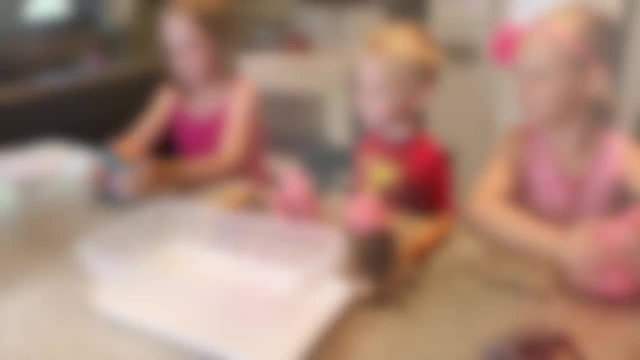 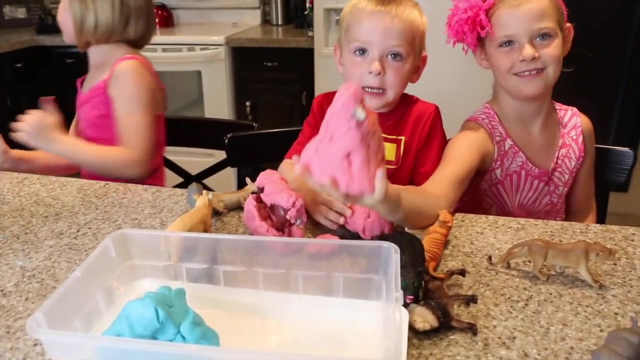 Only nine, nine, nine to five. When we're all done, we just store it in a plastic container with a lid and we can play next time. No, I'm not done. You're not done. Okay, Are you done? Adby, You got to take the animals out, if you're done.